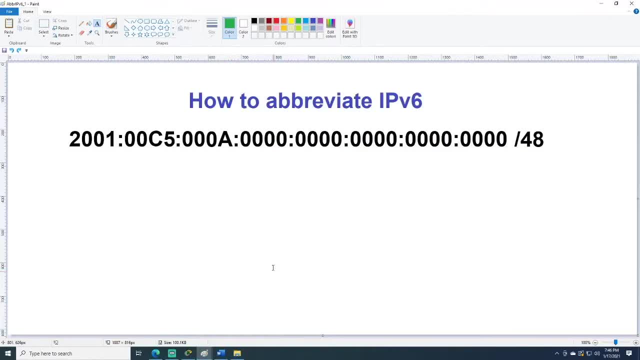 and try to abbreviate it yourself. Now let's check our work. In the first quartet we don't have any leading zeros, we just have trailing zeros. so this quartet must stay the same. In the second quartet, we have two leading zeros. 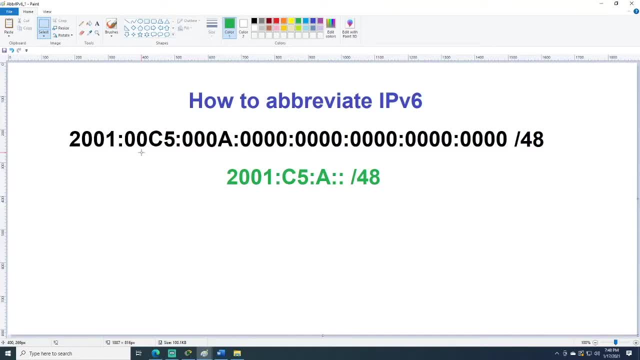 so we can get rid of those and represent this quartet as simply c5.. We have a similar situation in the third quartet, with three leading zeros and then the value a, So we can represent this third quartet as simply a. 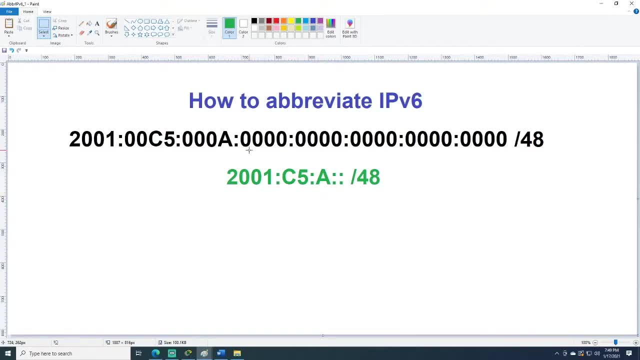 Following that quartet, we have succeeding quartets, five of them of all zeros, And so we can represent all five of these quartets with the double colon And, of course, finishing with our sider notation. Did you get the same result? 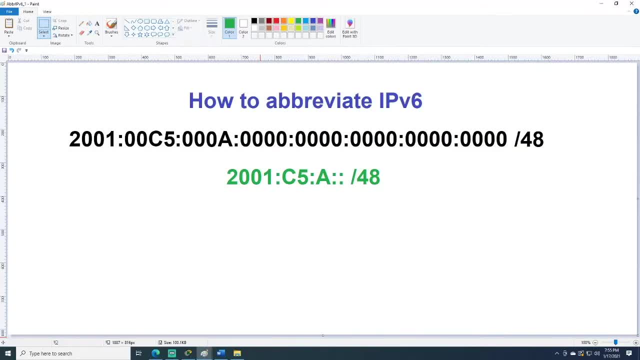 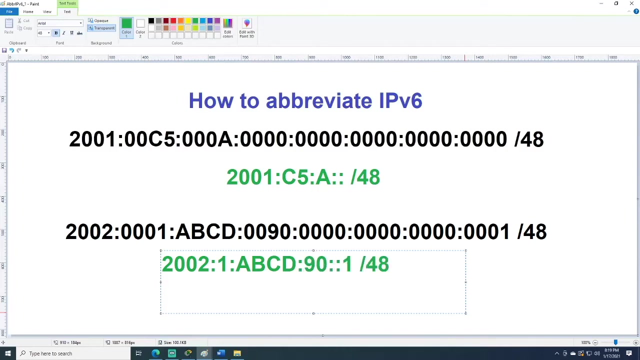 If you did, well done. But just to make sure we really understand this, let's try another one. Now let's check our work. We can see in this first quartet that again we have trailing zeros but no leading zeros. 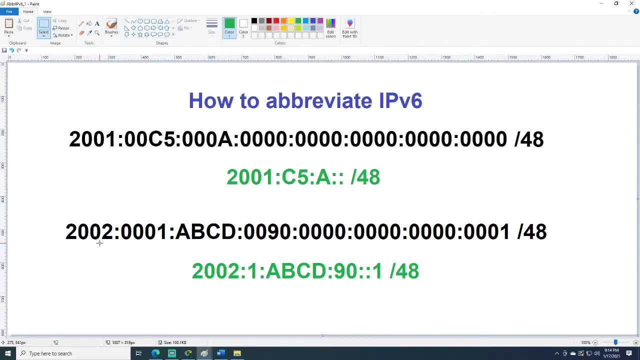 so this quartet must remain the same. In the second quartet we have three leading zeros, followed by a one, so that quartet can be represented simply as one. The third quartet has these four hexadecimal values of a, b, c, d. 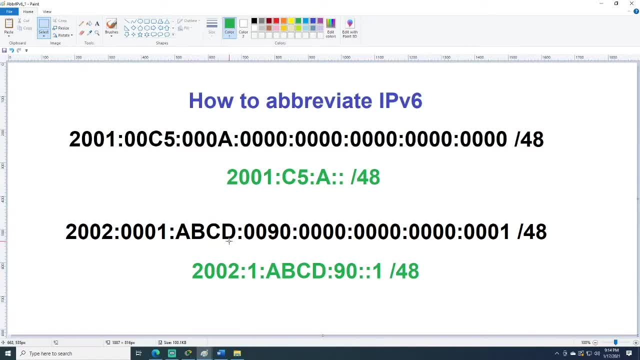 and so, with no leading zeros, this third quartet must stay the same. In the fourth quartet we have two leading zeros and one trailing zero. We can remove the two leading zeros, but the trailing zero must remain. so this fourth quartet can be abbreviated as 90..